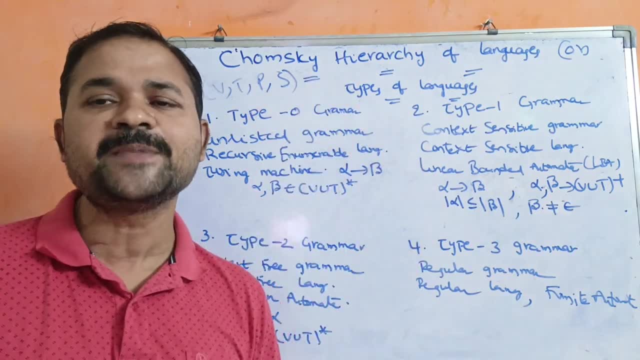 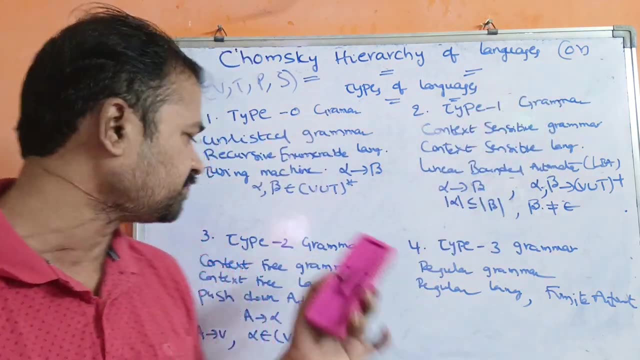 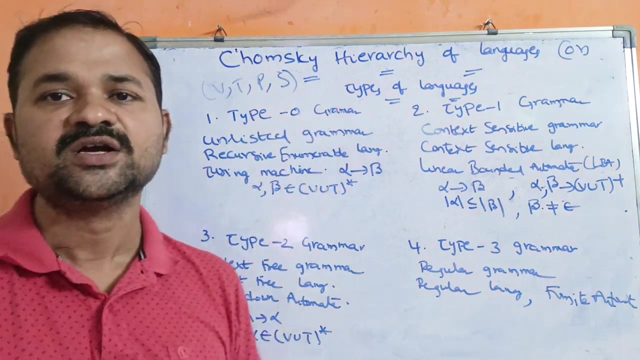 grammars And S represents start symbol Here. mainly we have four types of grammars are there. First one is type 0 grammar. Second one is type 1 grammar. Third one is type 2 grammar. Fourth one is type 3 grammar. So first let us discuss about type 0 grammar. Type 0 grammar. 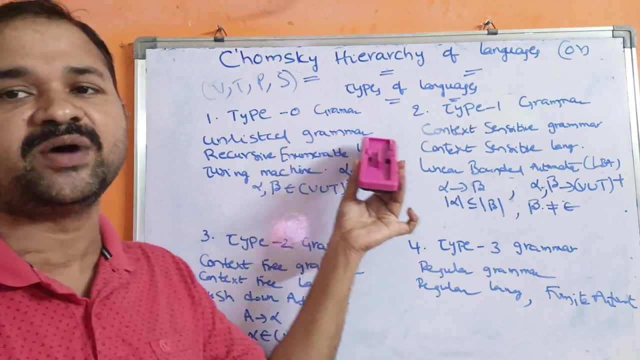 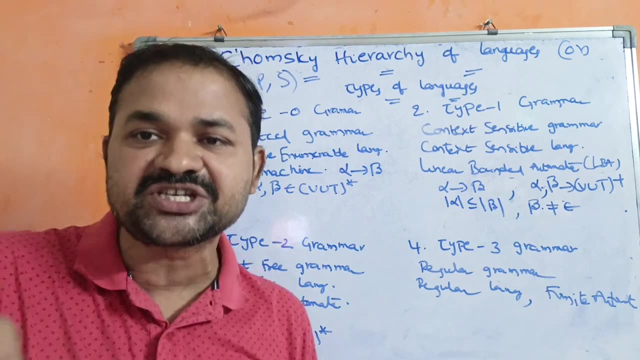 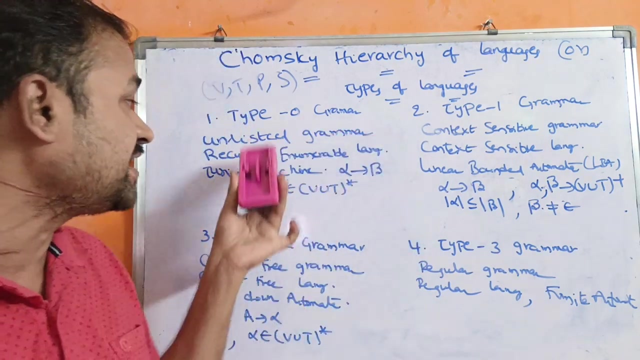 is also called as unrestricted grammar, So the name itself specifies the meaning: There is no restriction on the grammar. So there is no restriction on the left hand side of the production and right hand side of the production. An unrestricted grammar generates recursive enumerable language. In short, we can call it as REL. 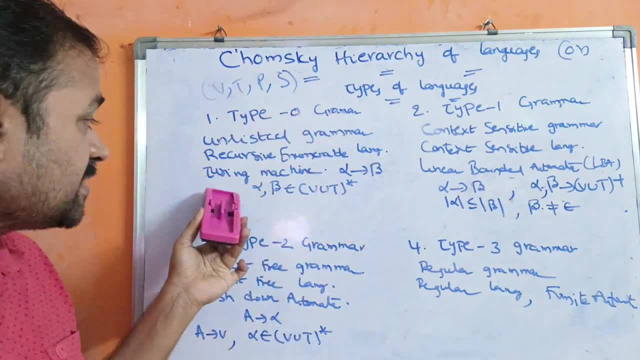 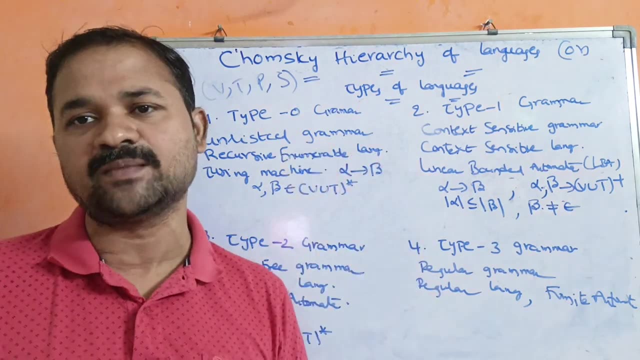 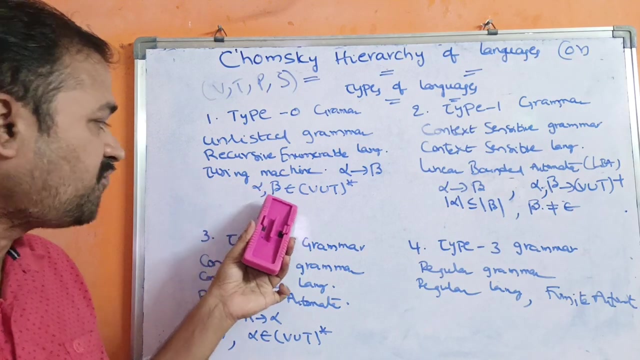 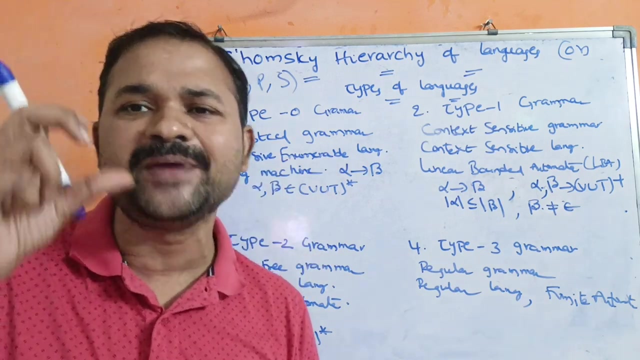 Recursive enumerable languages are accepted by Turing machine. Here the projections are represented in the form alpha implies beta. Alpha means left hand side of the production, Beta means right hand side of the production. Here alpha comma, beta implies belongs to V, union, T, whole star. That means alpha and beta is any combinations of non-terminals or terminals. 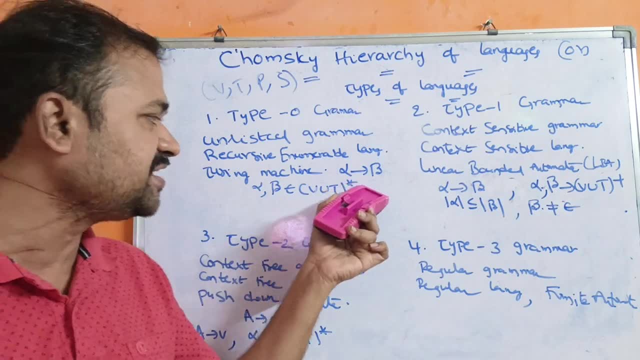 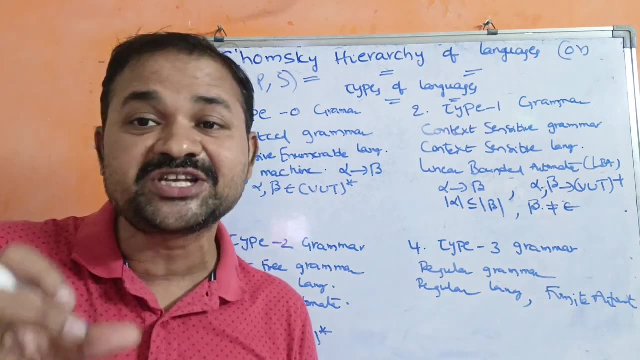 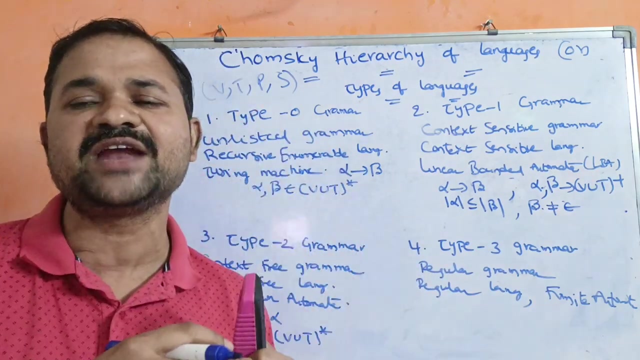 The supply of Turing people can also be nonsubstantiated or unobstantiated, or allicos or version of that product is also considered as unambiguous. E isn't sure but in the fact that an unab ص can have Siri in between n and R Inside. 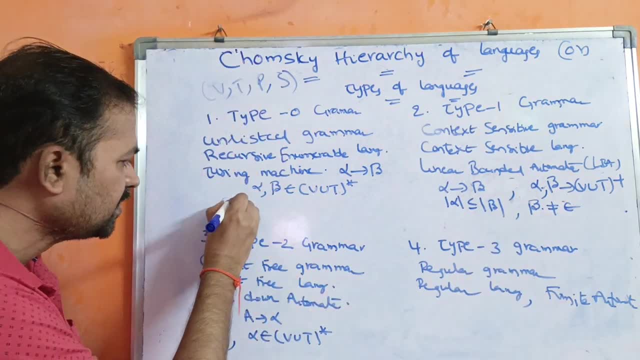 N is T for zero. nearest-to-neo mean this N sample of a. So even the planet God can create a friendless mind, But they don't discuss about it. The option of theółi and the' tormentoraries points out thus: Ab implies b. So we have only onelas, Trib temples並fitna, and We have 0 равно term. So here in this example starting is .2V and 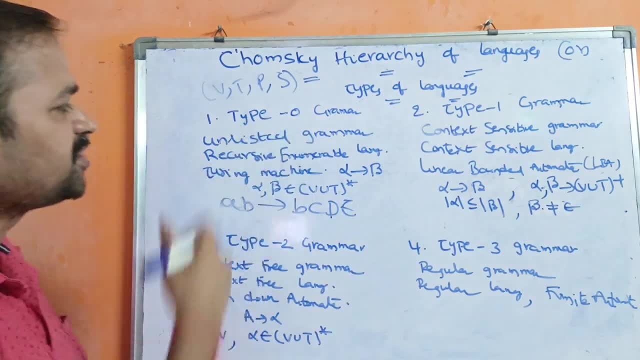 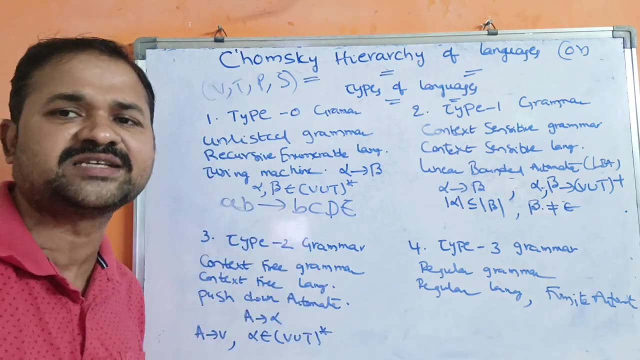 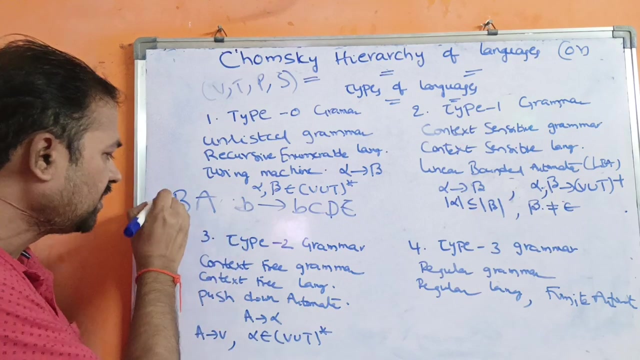 c, d, e. so this is nothing but this production, only recursive enumerable language production only. why? because we can have any number of non-terminals and terminals. so we can write some some non-terminals before this one or between this. this is also a production, okay, so we can write any number of. 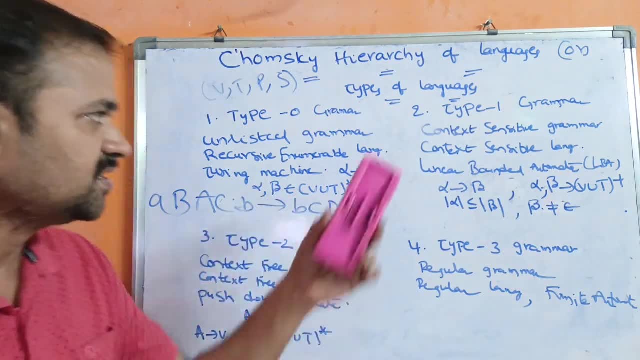 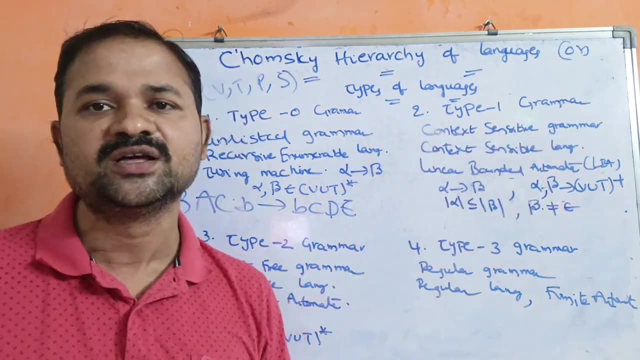 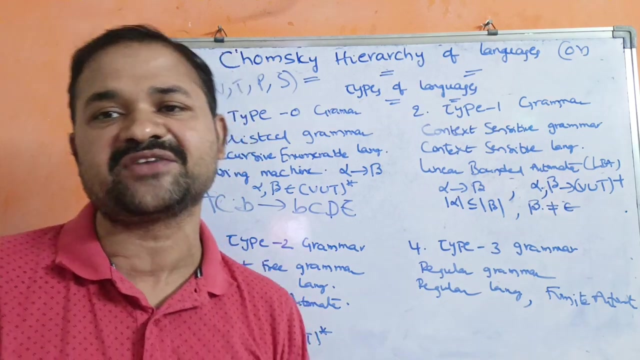 terminals and non-terminals in lhs and rhs. now let us see about type 1 grammar. type 1 grammar is also called as context sensitive grammar, in short we can call it as csg, and context sensitive grammar generates context sensitive language, csl. context sensitive languages are: 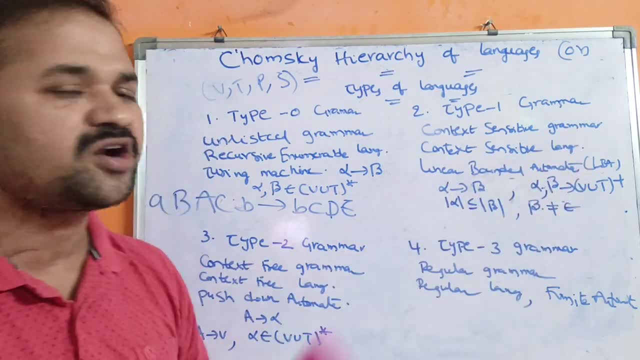 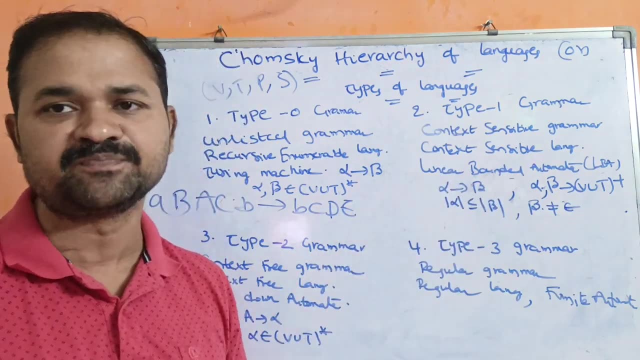 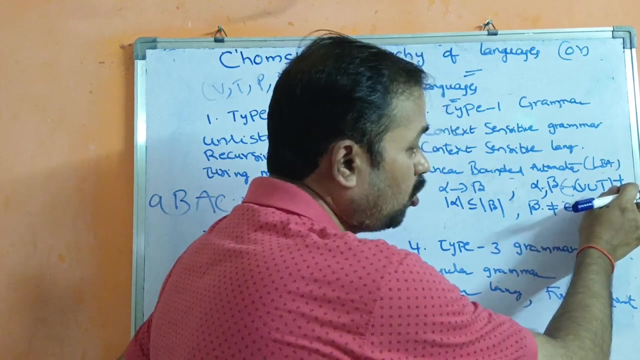 accepted by linear bounded automata. in short we can call it as lba. here also the productions are represented in the form alpha implies beta, but here alpha and beta belongs to, belongs to you, v union, p, 4, power, plus. So plus means minimum one occurrence, minimum one occurrence. That means 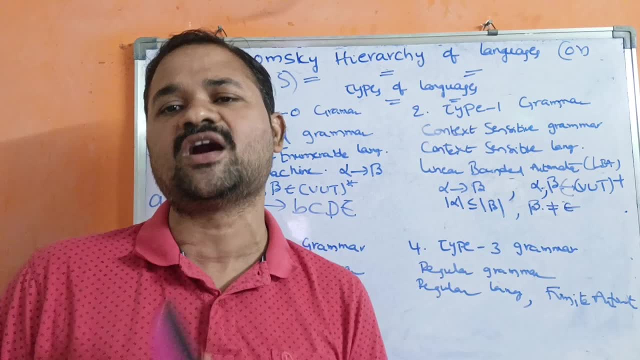 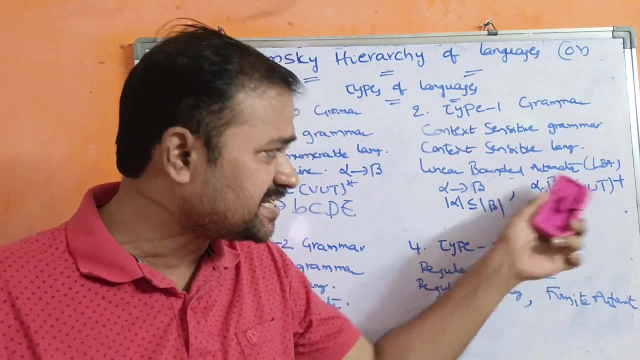 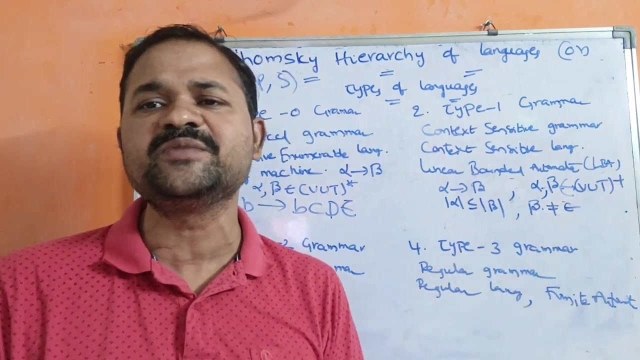 epsilon is not allowed in LHS and RHS, So we have. it is also a combination of here: RHS is left LHS and RHS left hand side of the production, and right hand side of the production is also a combinations of non-terminals and terminals, but minimum one occurrence. So that is why we use. 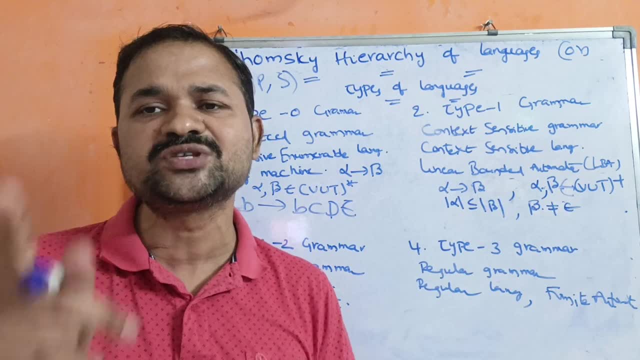 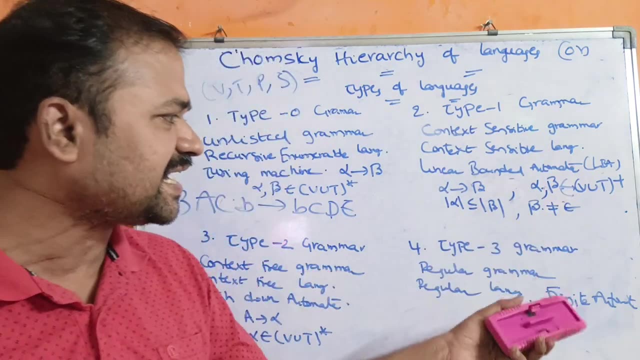 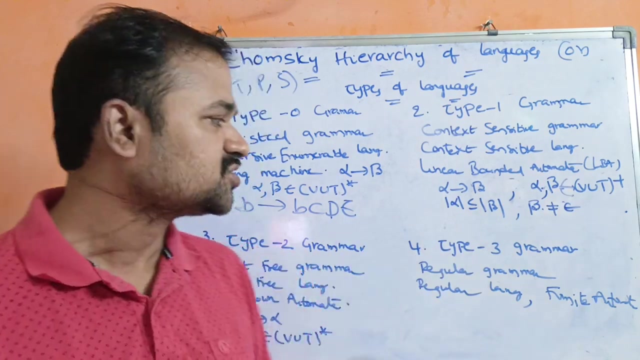 plus. Plus means minimum one occurrence. So we have to use minimum, minimum one non-terminal or terminal in LHS and RHS, minimum one occurrence. Let us see the condition here: mod alpha is less than or equal to mod beta. So that means here mod represents length, So length of the left. 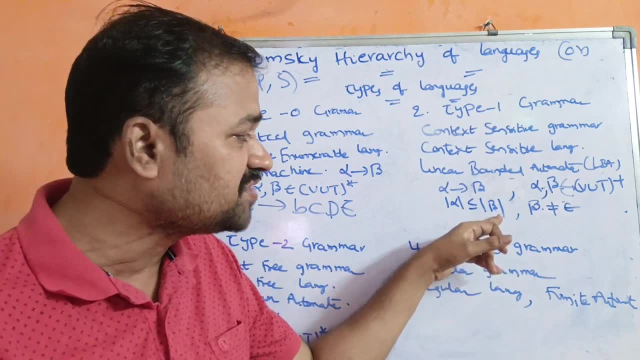 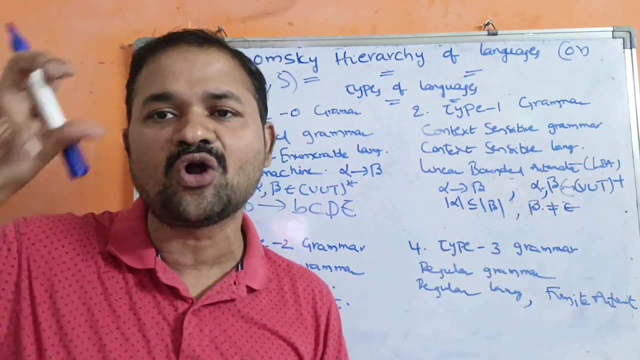 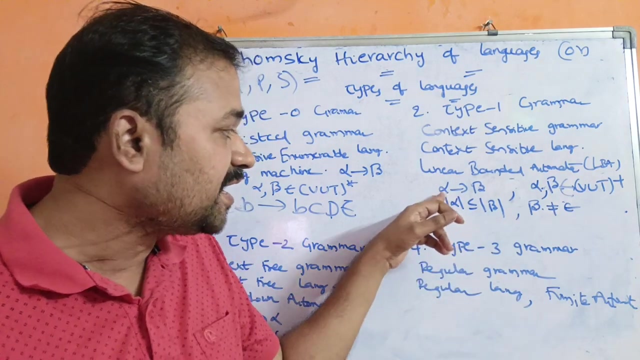 hand side production must be less than or equal to length of the right hand side production. And one more condition: is beta not equal to epsilon, So right hand side should not contain epsilon. Right hand side should not contain any epsilon. And one more condition here is here left. 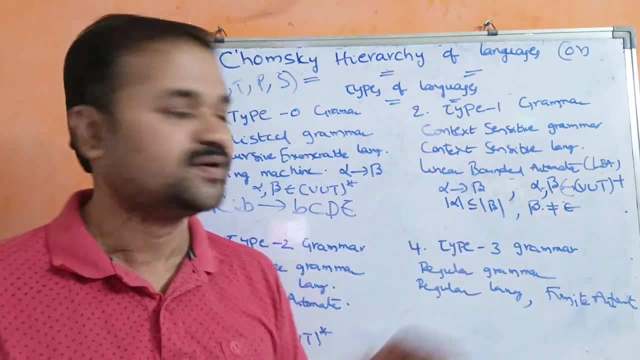 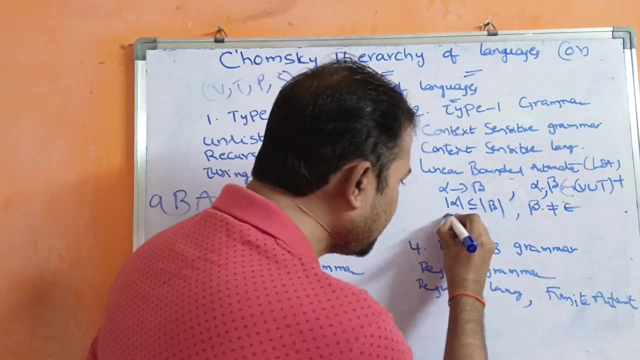 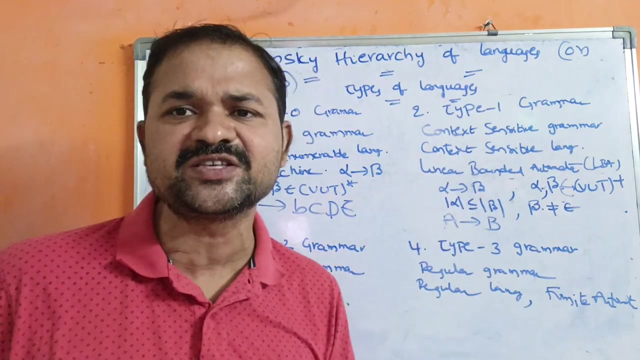 hand side production should contain minimum one non-terminal LHS. left hand side of the production should contain minimum one non-terminal. Let us see some examples. A implies B. A implies B Is it. is it a context sensitive language production? A implies B Here. LHS contains one non-terminal. So 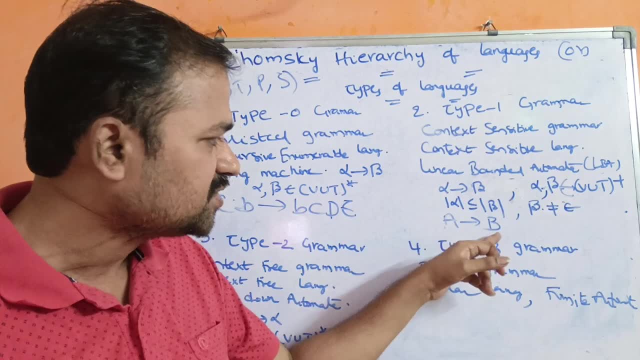 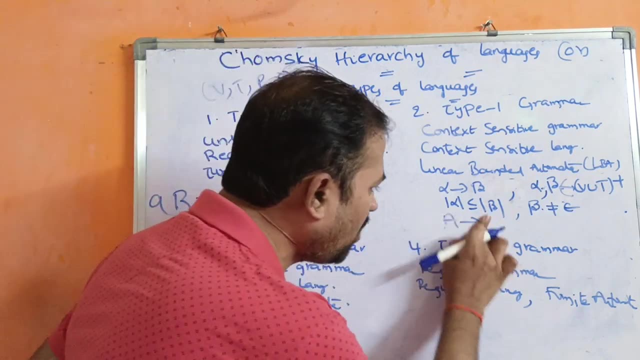 there is no problem. And what is the length of the CA1.. So what is the length of the B1?? So 1 less than or equal to 1.. So this is a valid production. Next let me have A implies epsilon. Is it a valid production? No, 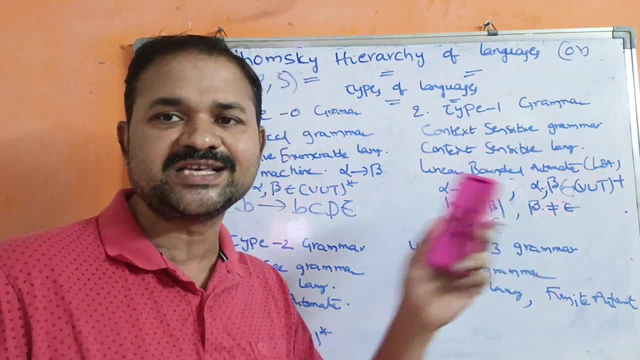 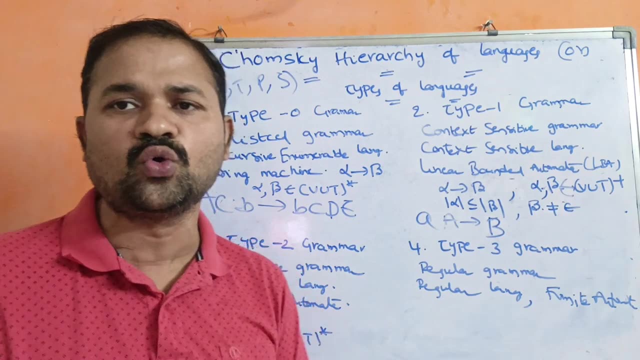 Why? Because RHS should not contain epsilon. This is not a valid production. Next, AA implies B. Is it a valid production? No, Why? Because what is the length of LHS2? Length of RHS1.. 2 less than. 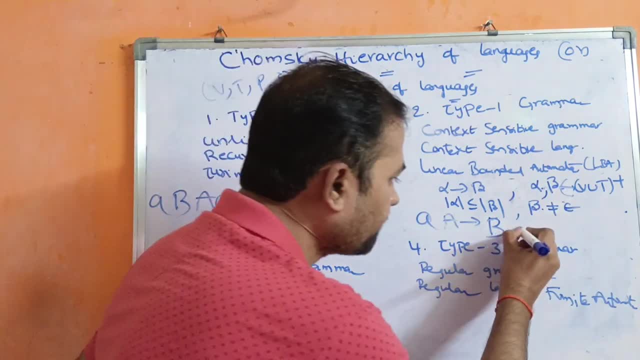 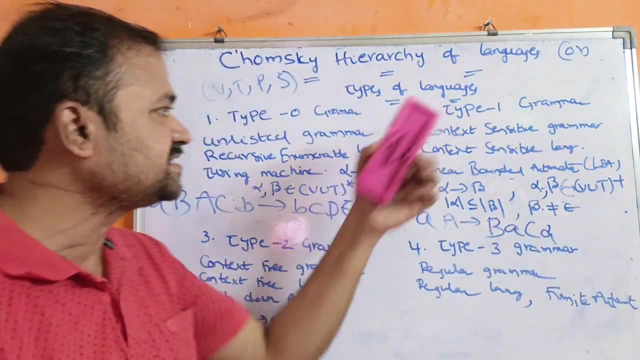 or equal to 1.. this is not a valid production. next, b ac. is it a valid production? yes, why? because 2 is less than or equal to 4. okay, so this is about type 1 grammar. now let us see about type 2 grammar. type 2 grammar. 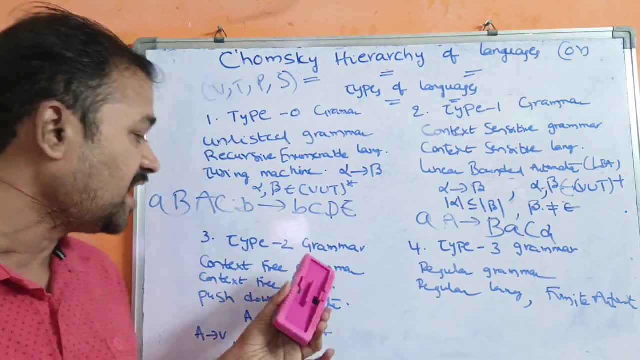 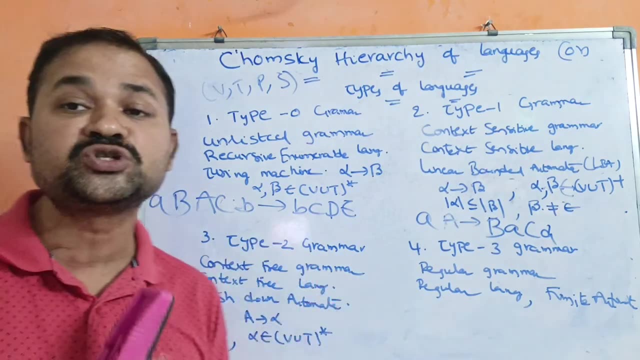 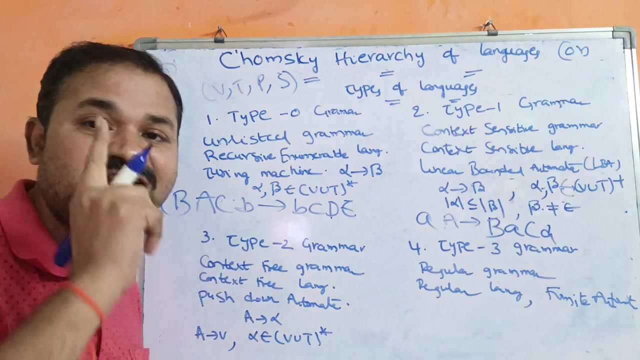 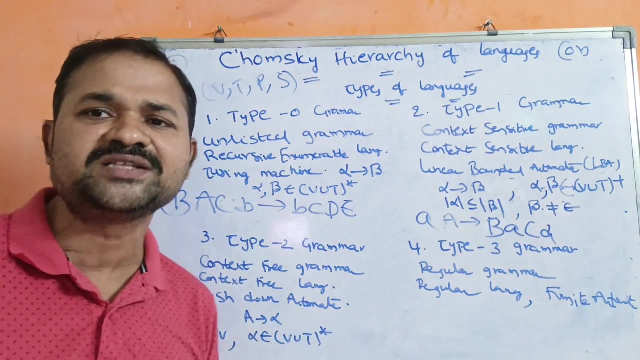 can also be called as context-free grammar, cfg, and context-free grammar generates context-free language. context-free languages are accepted by pushdown automata. here the projections are represented in the form: a implies alpha, where a is a single non-terminal. where a is a single non-terminal, whereas alpha is a combinations of non-terminals and terminals. we can use zero. 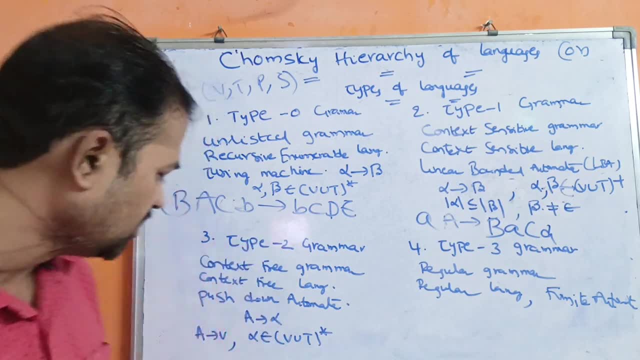 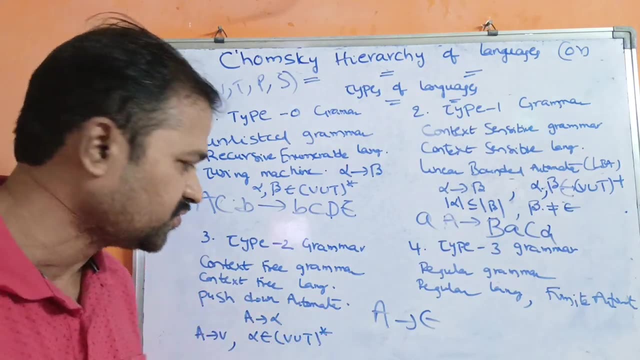 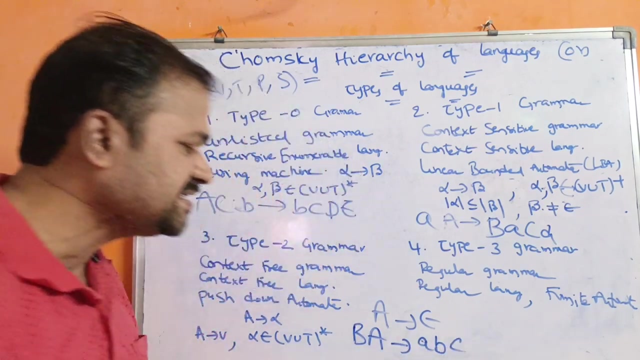 occurrences also. that means epsilon can also be allowed. so let us take an example: a implies epsilon, so this is a valid projection. why? because here rhs may contain epsilon also. next next: ba implies, ba implies abc. is it a valid production? no, why? because here the left hand side should contain only one non-terminal. 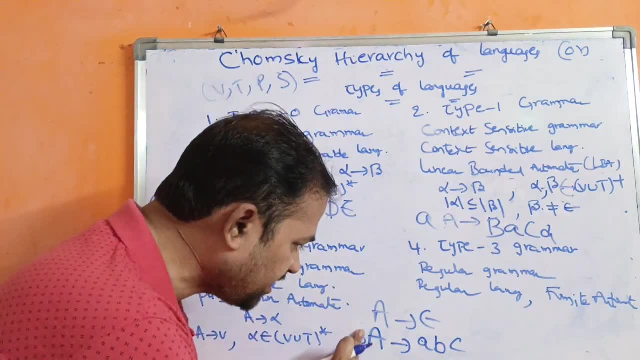 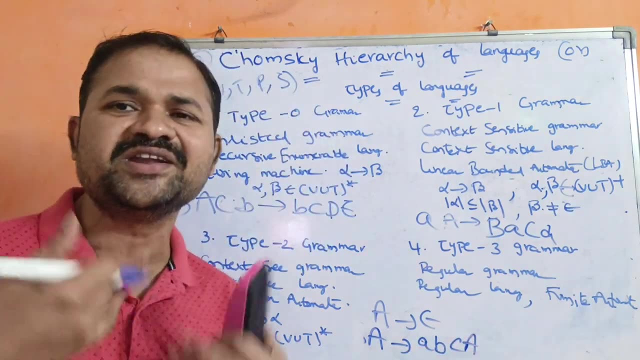 but here we have, here we have two non-terminals. it is not a no. is it a valid production? yes, it is a valid production. is it a valid production? yes, why? because rhs may contain a combinations of non-terminals and terminals. there is no problem. now let us see the last grammar, that is type 3. 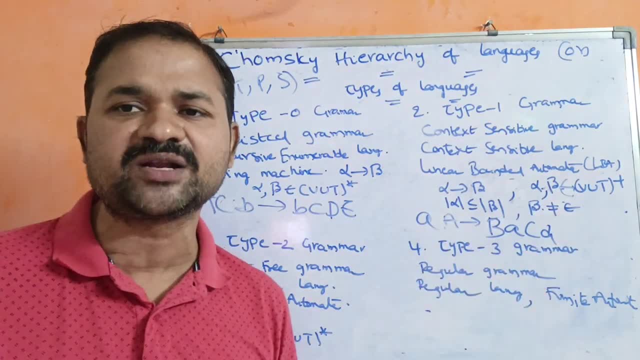 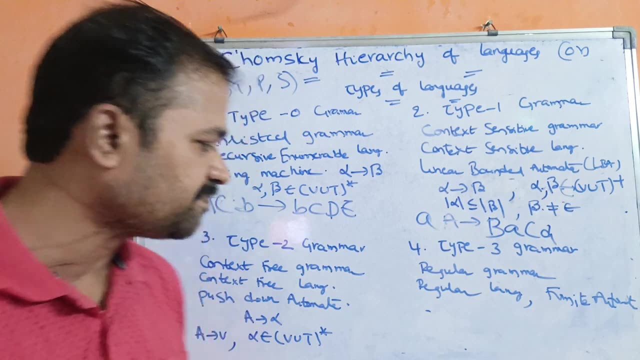 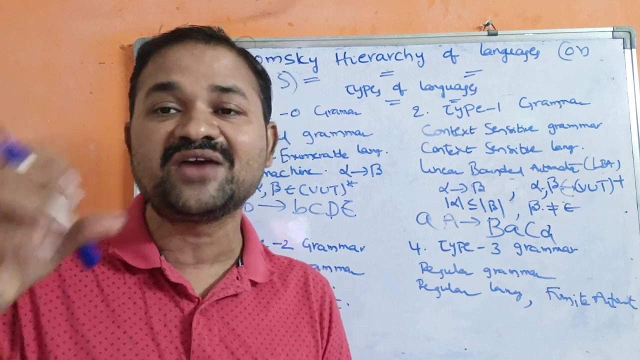 grammar. type 3 grammar is also called as regular grammar. regular grammar generates regular languages. then regular languages are accepted by finite automata. okay, here we have two types of regular grammars. are there left linear grammar as well as right linear grammar? so left linear grammar means: 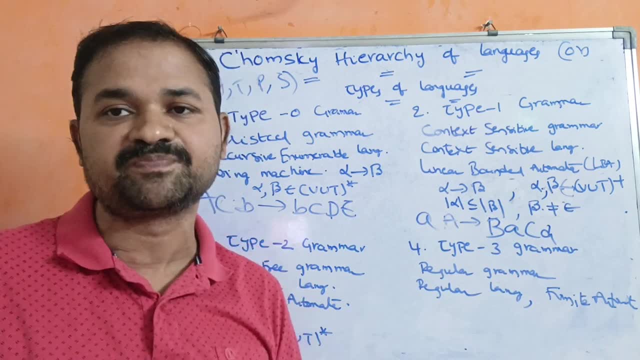 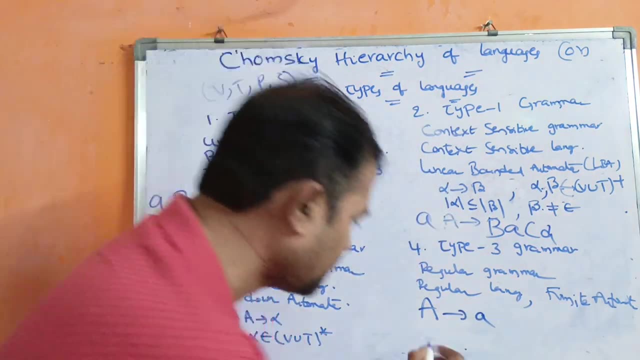 the left hand side production must be, but starts with non-terminal. so let me have a left. linear grammar means a implies here, so we can have a single terminal, there is no problem. so a implies this: right in this right hand side, production in this production, left hand side.